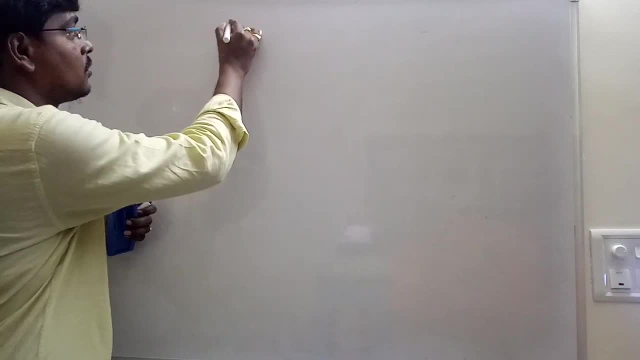 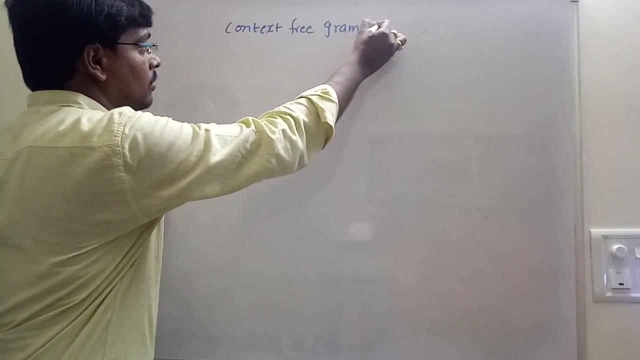 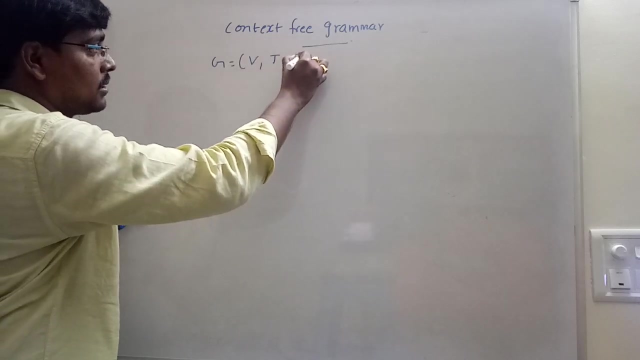 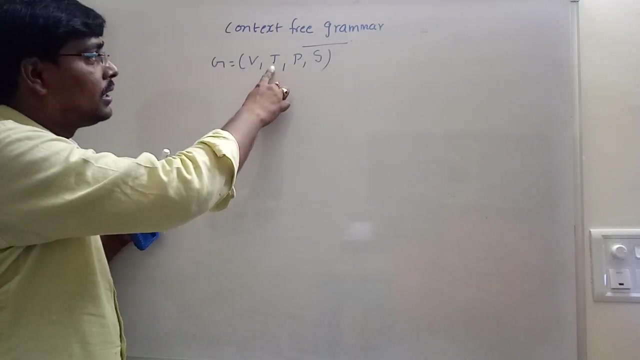 Hi friends, today's topic is context-free grammar. Consider a grammar: g is equal to v, t, p. s is a context-free grammar. v is the set of non-terminals, t is set of terminals, p is the productions, s is the start symbol. 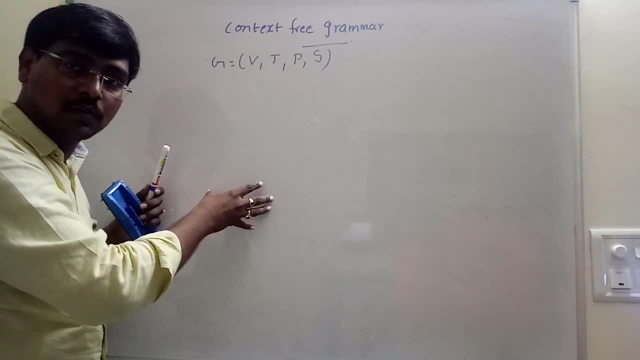 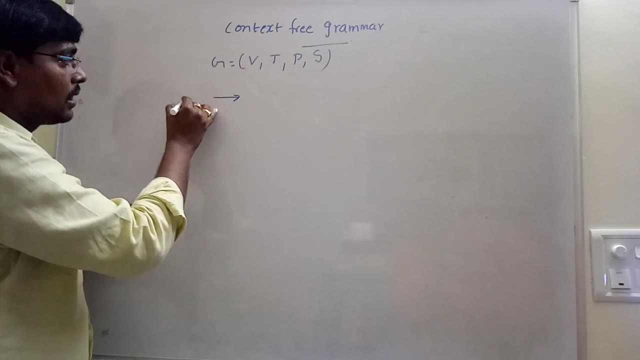 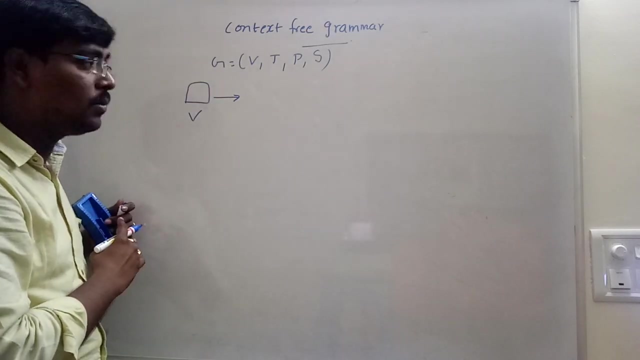 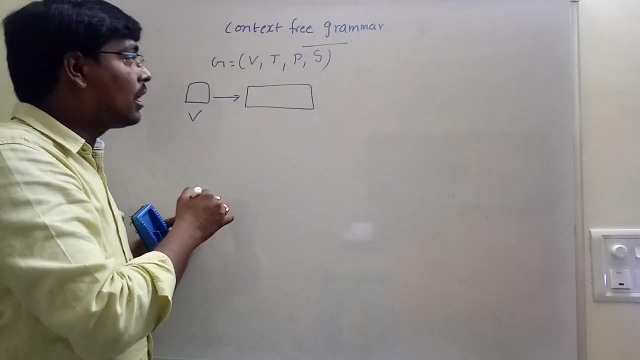 Suppose, if these terms become a context-free grammar, we will have to follow some of the rules. So simply, the rules are: the left side of the production must be a non-terminal and right side of the production is either epsilon or a combination of terminals and non-terminals. 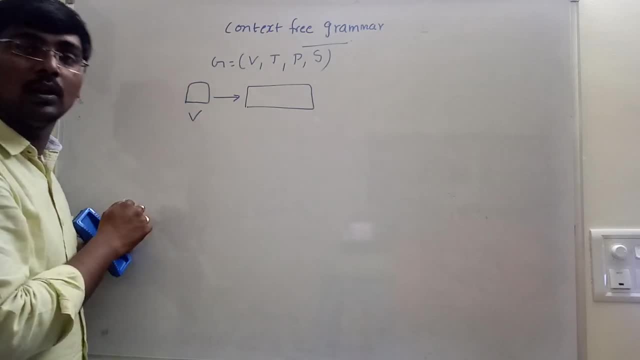 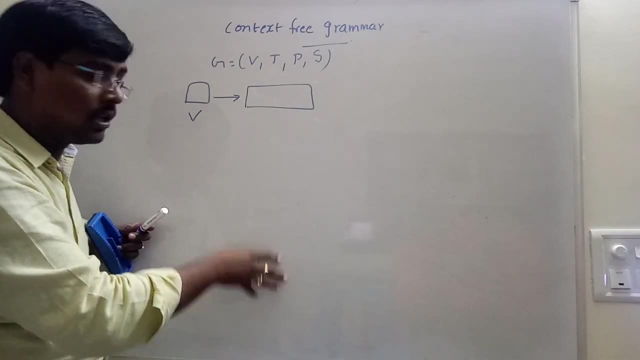 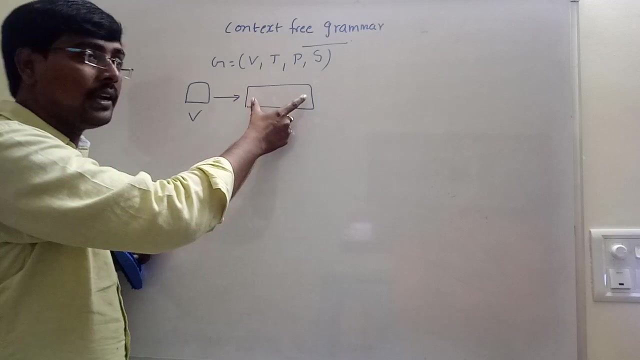 And left side must and should continue. There is only one non-terminal variable. So what is the meaning of production means In the process of derivation, whenever a variable that is a non-terminal appears, that is replaced with the entire string placed on the right hand side. 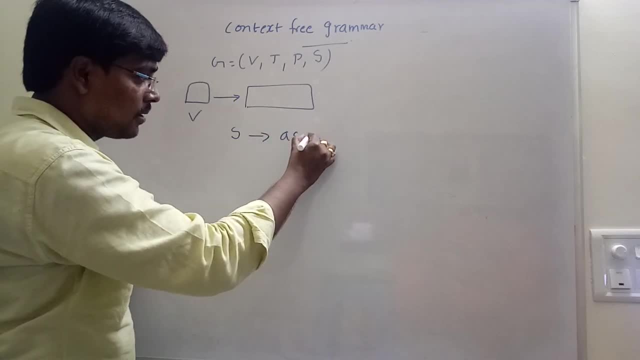 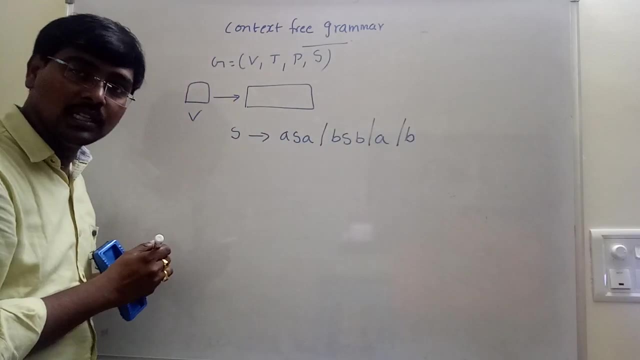 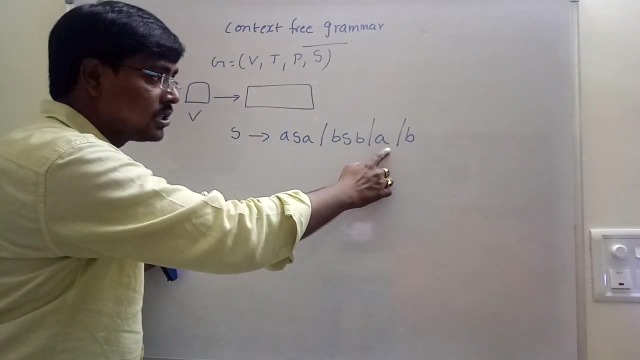 For example, s is equal to a, s, a or b, s, b or some a or b, For example. this is a context-free grammar. Here s tends to a, s a, s tends to b, s, b and s tends to a, s tends to b. 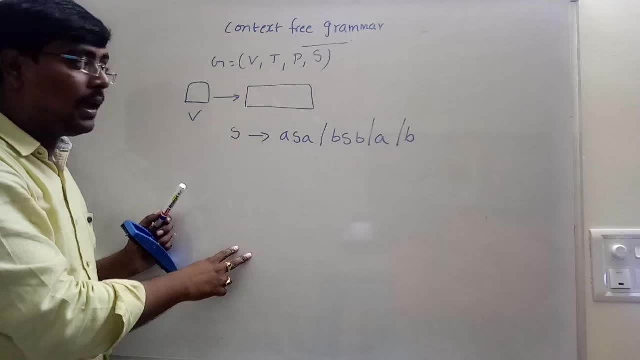 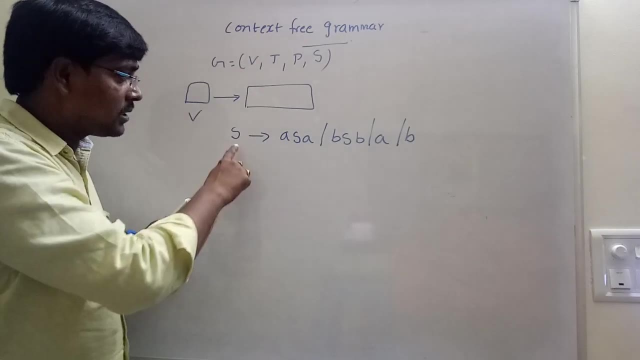 are the four productions. those are represented by p And the terminals, that is small letters. a, b are represented by t, The capital letters, so only s that is represented by v. Here s represents starting symbol. Suppose we have more than one production. 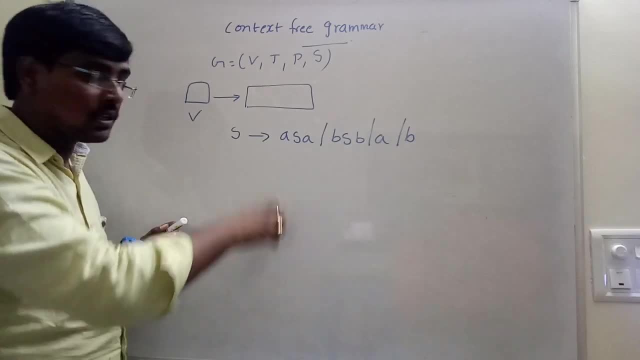 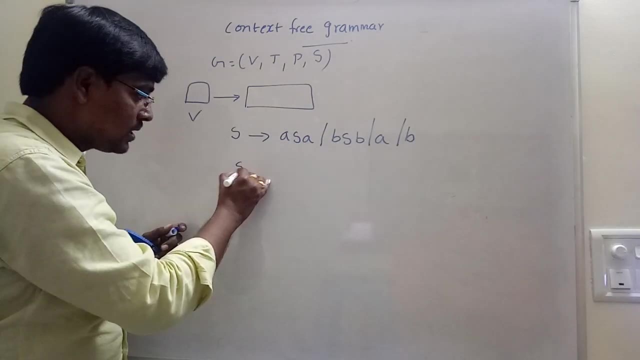 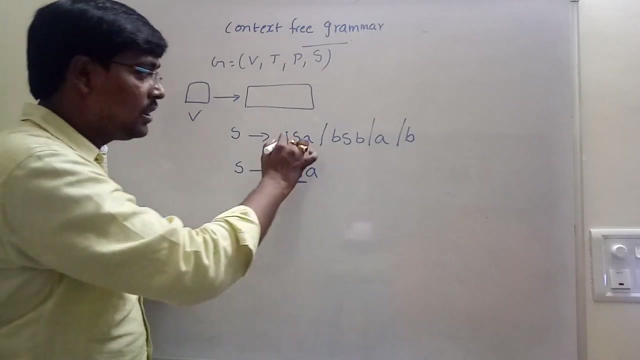 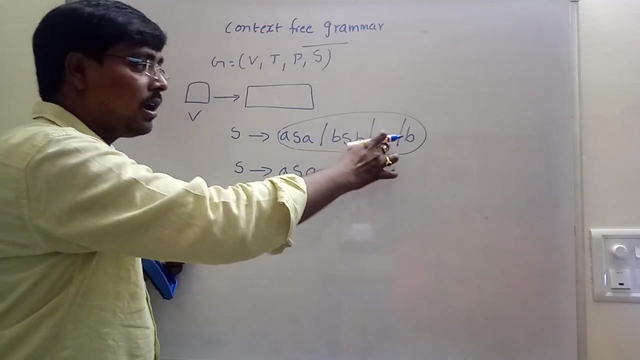 Suppose with different names The first 2 productions: The first production, First, Stefan. first variable is the starting symbol. so to derive a string: suppose s tends to a s a. whenever s appears, s is replaced with any of these four terms. suppose s is replaced with either a, s, a or b, s b or a or b, depending on our string. for 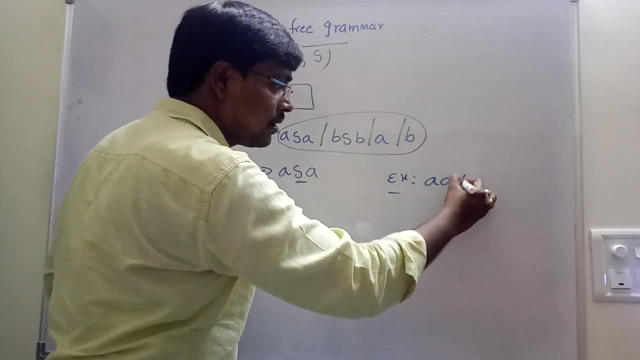 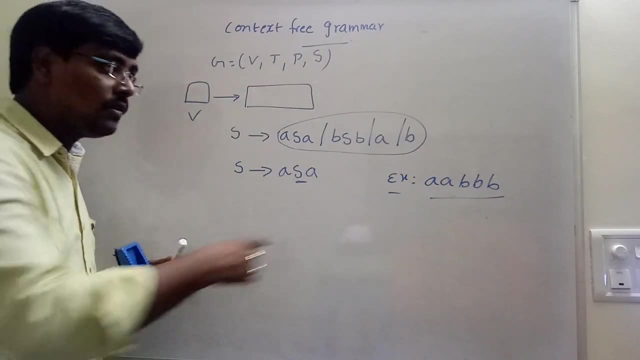 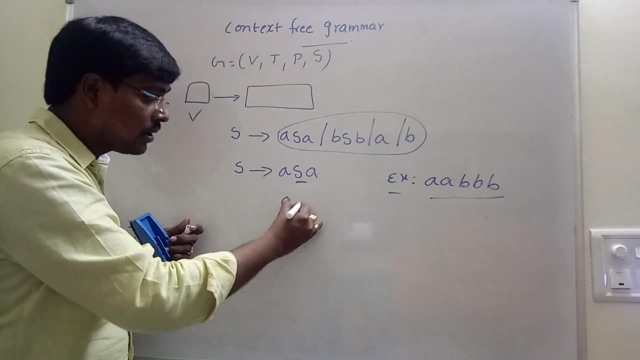 example, if our string is aa, b, b, b. suppose if our string is in this format: aa, b, b, b, check whether it is possible to delete the string or not. suppose the first string is a sa, a, SA, no, this, yes is requests me. suppose second character is also in second, and then 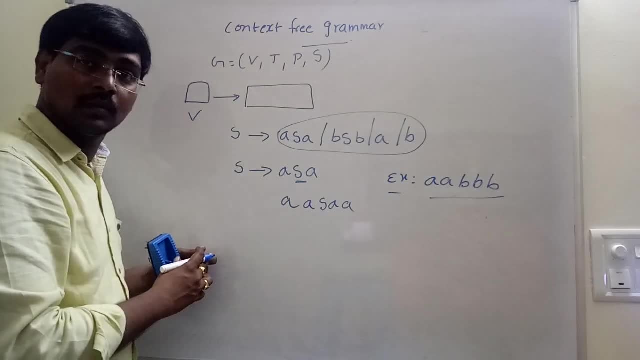 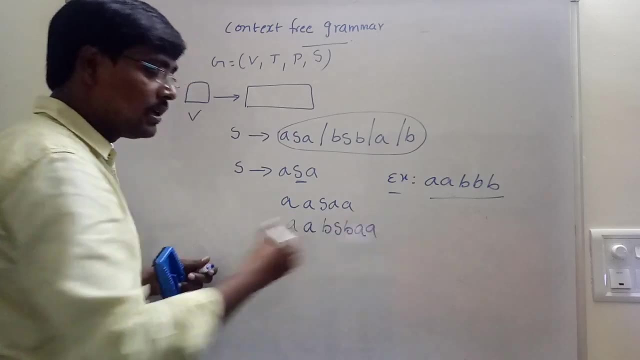 replaced with as aio. now yes is replaced with some angry s. the catcher is always forgot. the between the say of can be translated as: but let's say a now yes is correct me, right now it's another. we print place with some any other character: a, a, b, s, b, a, a. check the possible cases. for all the cases, the last. 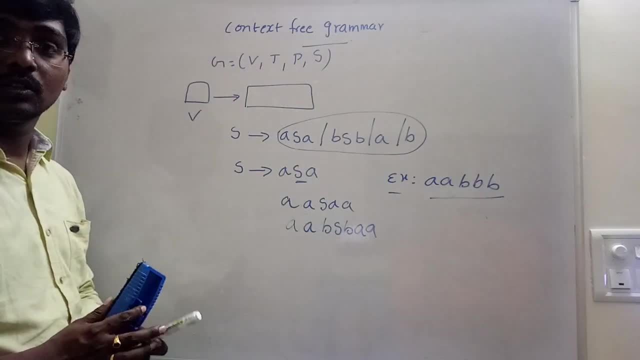 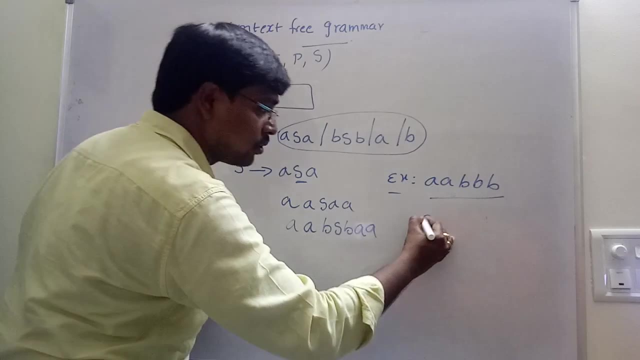 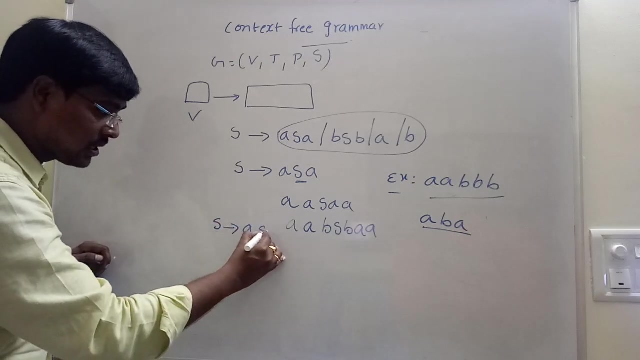 character is b, it is not possible to derive the last character. suppose if last character is b, first character a. so this string is not possible. suppose check one more string: a, b, a. this is a possible or not? so s tends to a, s. a suppose if this s is replaced with a letter: b a, b a. 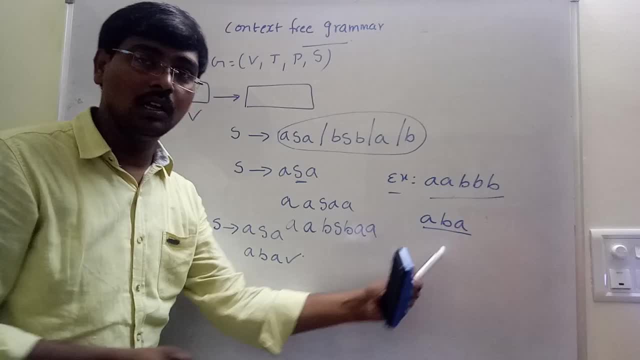 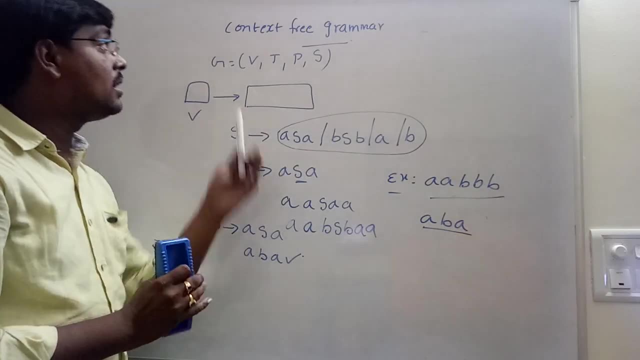 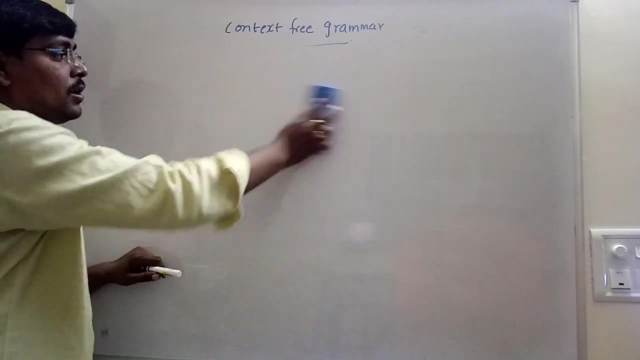 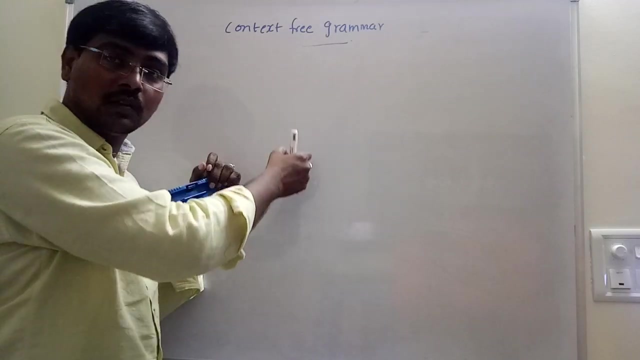 the string is derived based on our string. we are replacing this non-terminal value with any of the production right hand side production. this is a context-free grammar. so to derive a string here. the main point is to derive a string. we are following some procedure, you. that is called derivation. derivation means a sequence of steps taken to derive a string, so 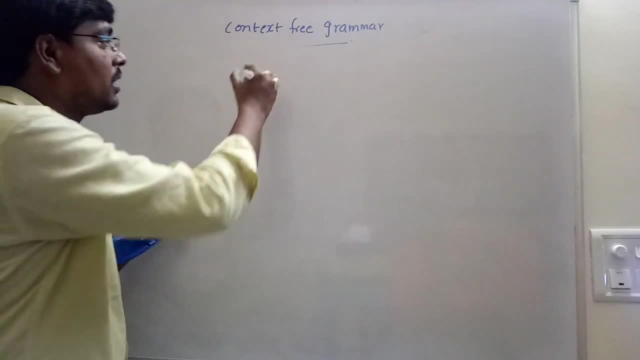 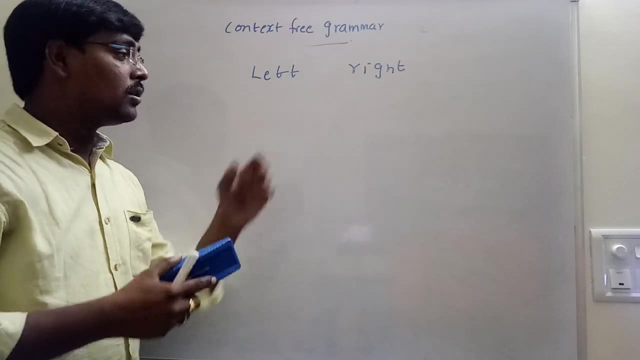 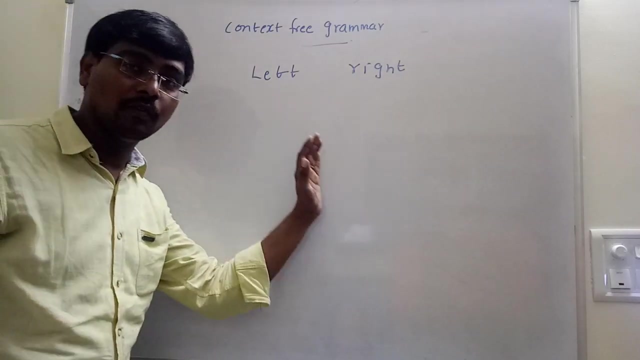 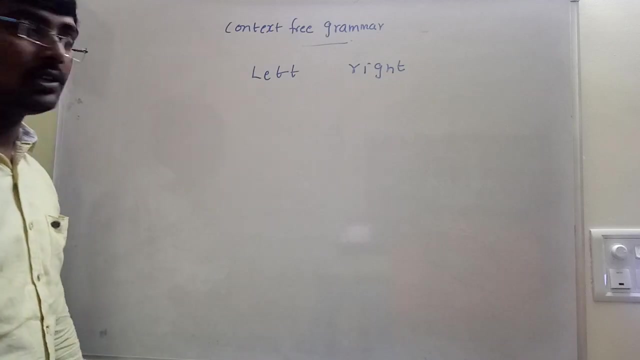 derivation is of generally two types: either leftmost derivation or rightmost derivation. the name itself says during the process of derivation: first, if left to side variable, that is scanning is from left to right and the replace of the variable is also from left to right. that is leftmost derivation. scanning is from right to left and replacement of the 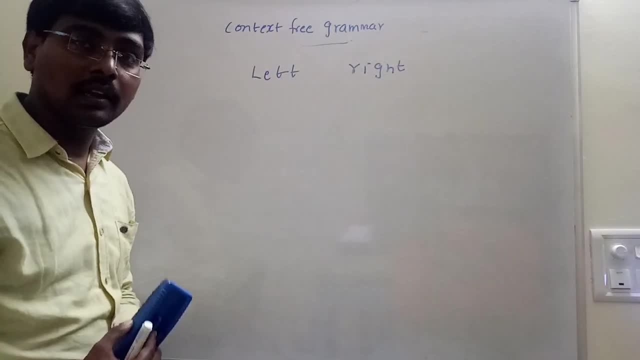 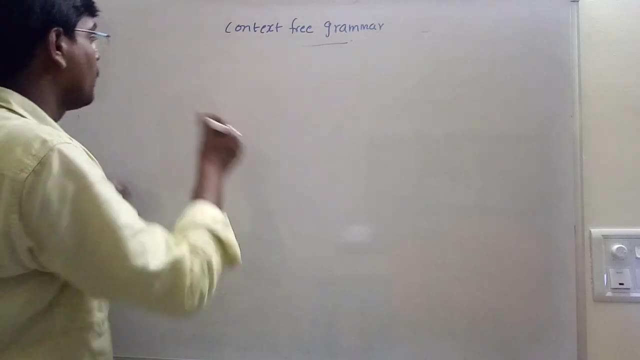 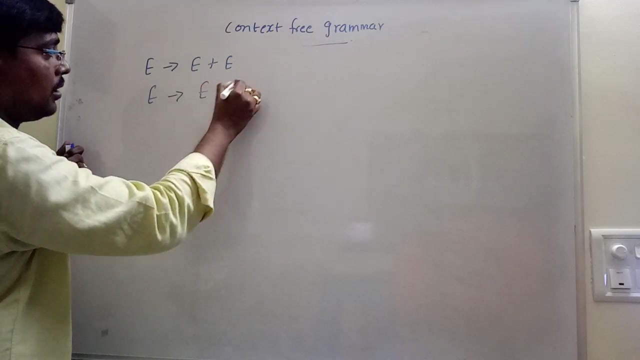 variable is also from right to left. that is called rightmost derivation. now consider an example to check leftmost and rightmost derivation. suppose the string e is equal to e plus e. e is equal to e into e. suppose e is equal to id. this is the grammar for this grammar we are based on this. 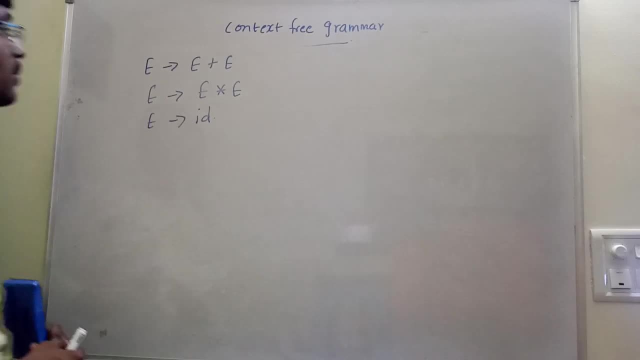 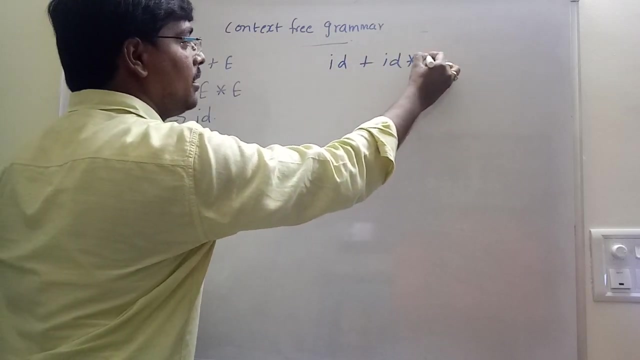 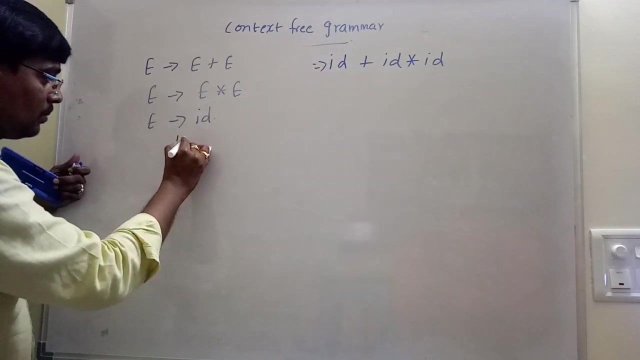 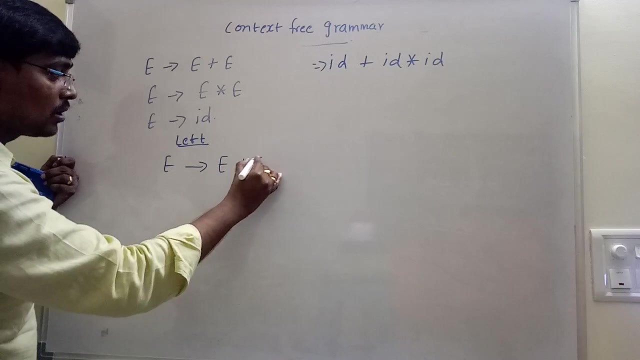 grammar. we are performing leftmost derivation and rightmost derivation. For example, id plus id into id. This is the string we want. This is the string we want First to perform leftmost derivation: First to e, equal to e into e. sorry, e plus e. Now, first to e is replaced with, so. 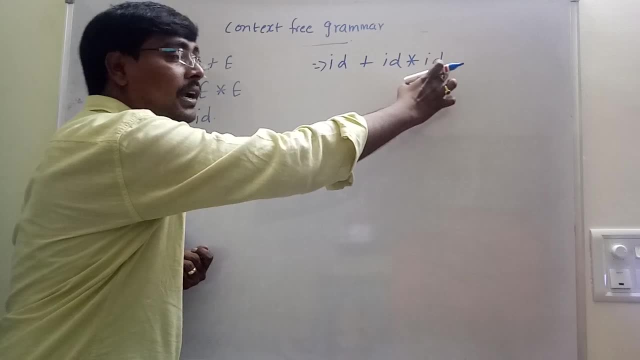 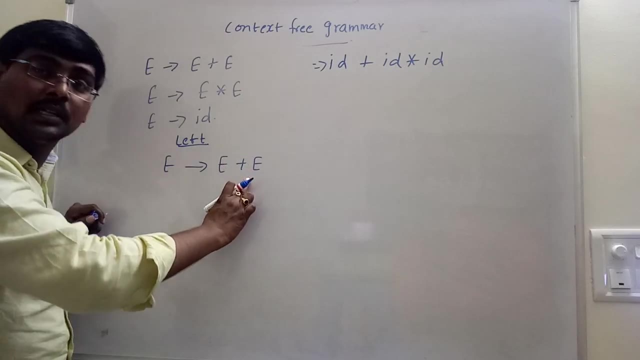 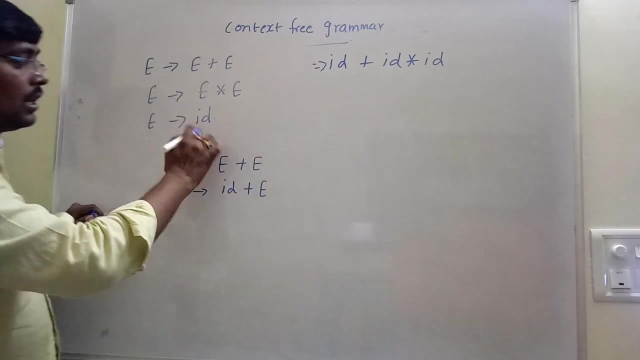 check the pattern. So id plus id into id. So first to: after replacing one letter, the next symbol is compulsory: a plus o. So e is replaced with id plus e. Let's see Leftmost derivation scanning from left to right. Now id plus. Now the next two pattern. 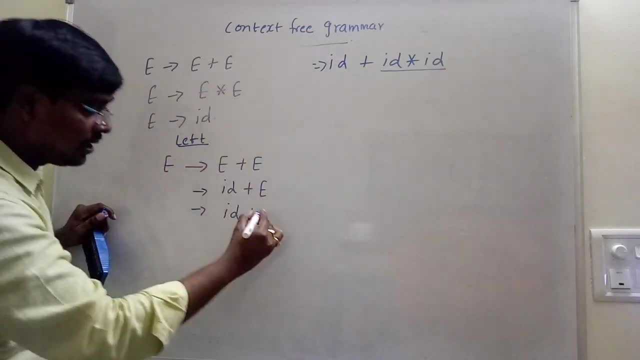 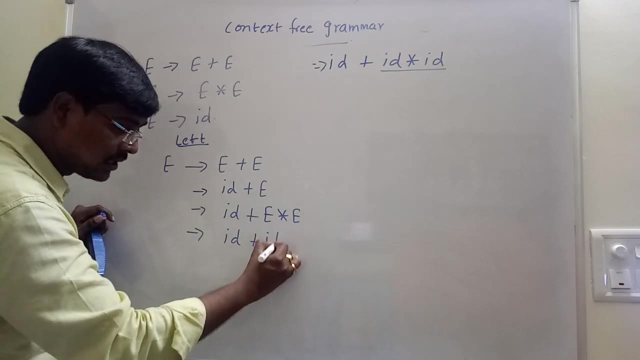 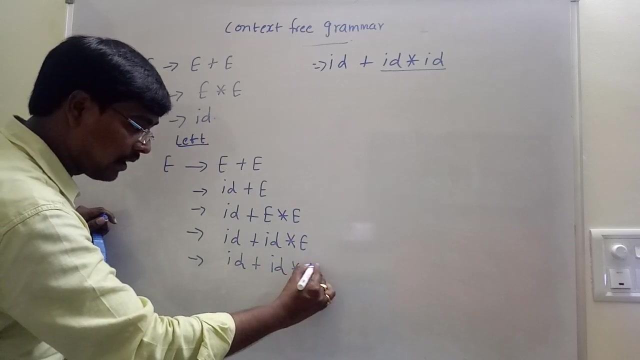 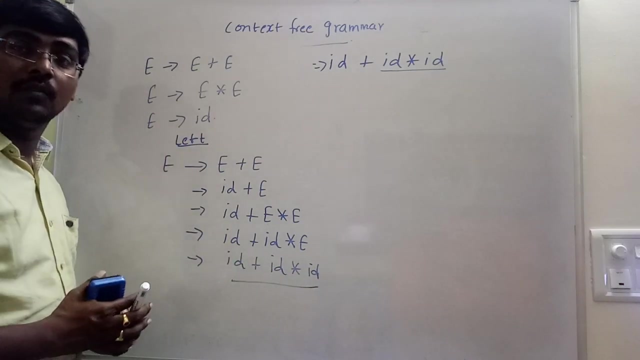 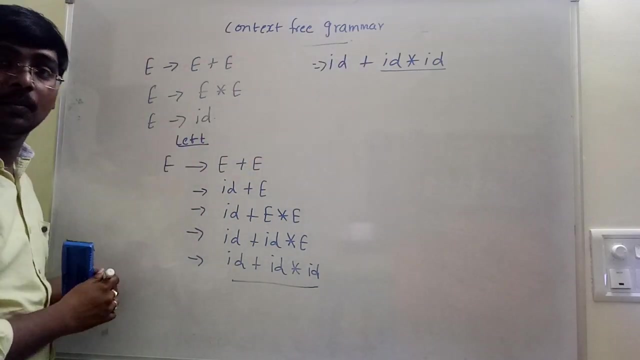 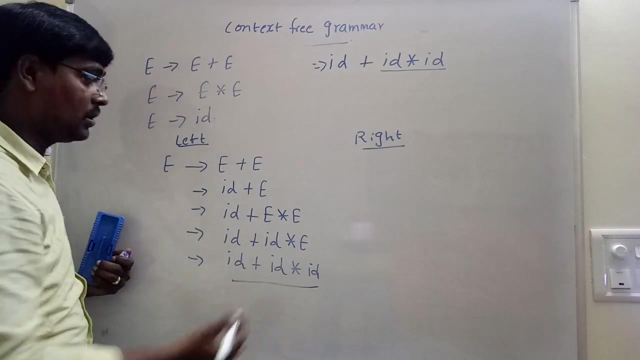 is id into id. That means the replace with e into e. Now id plus This e is replaced with id. In the next step, id plus id into id. This is the pattern we are getting id plus id into id. Moving on to letter: 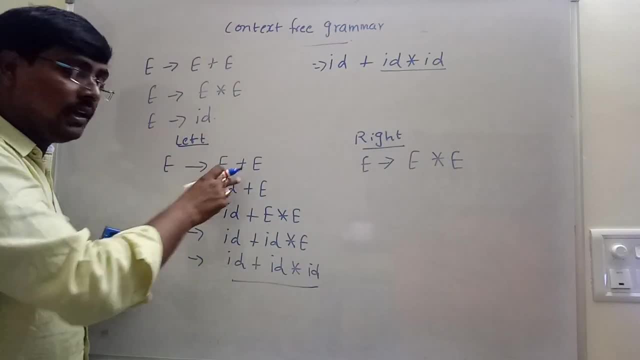 e into e To стало. a rightmost derivative string is believe to be a leftmost string. This is what we are getting. There are no leftmost string in the rightmost string. We are generating a leftmost string. Similarly for that same string with the same context. 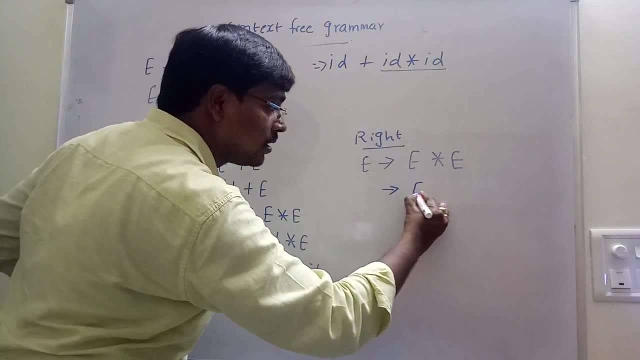 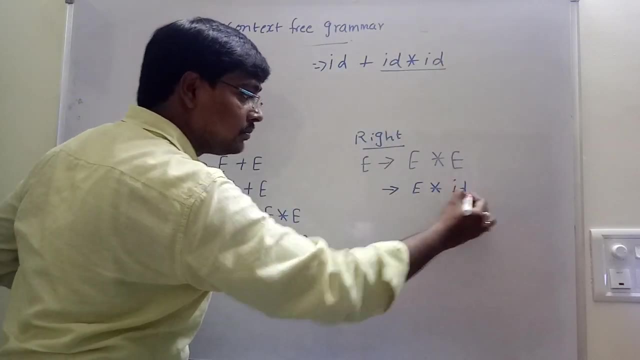 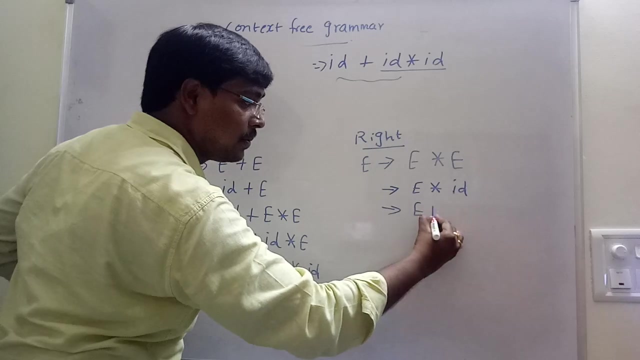 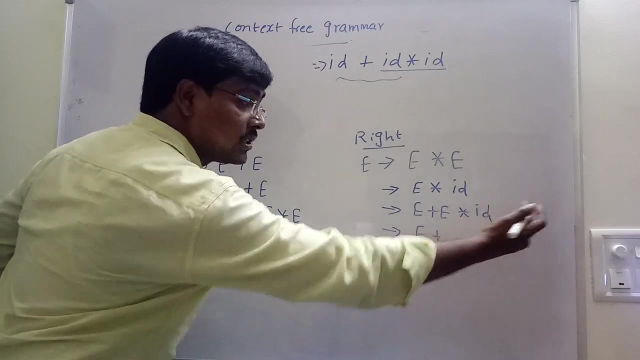 this e. First replace this e, Suppose e into, so this e is replaced with id. In the next step, replace this e. This e is replaced with. to get this expression: replace with e plus e into id. Now e plus replace- so scanning from right to left- this e id into id. 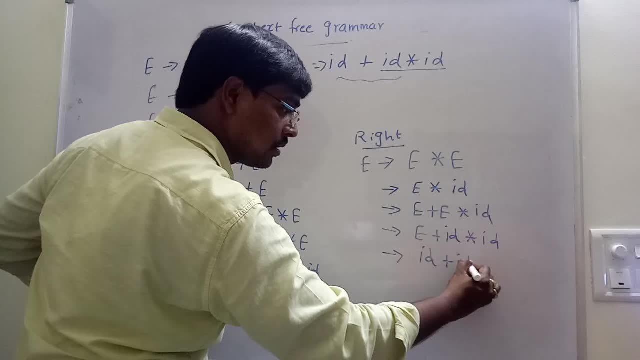 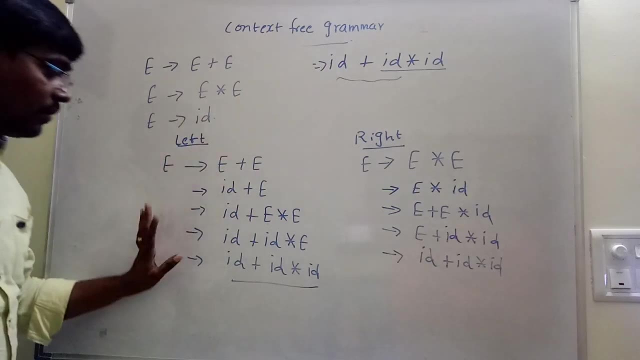 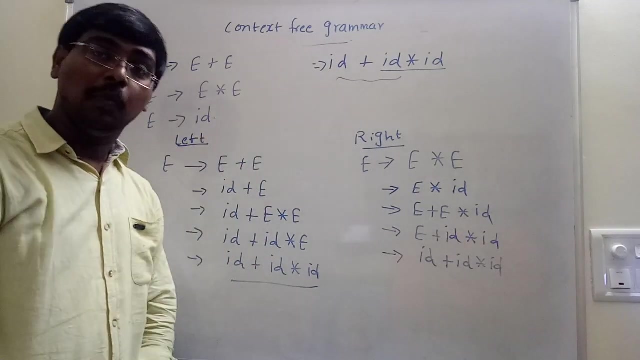 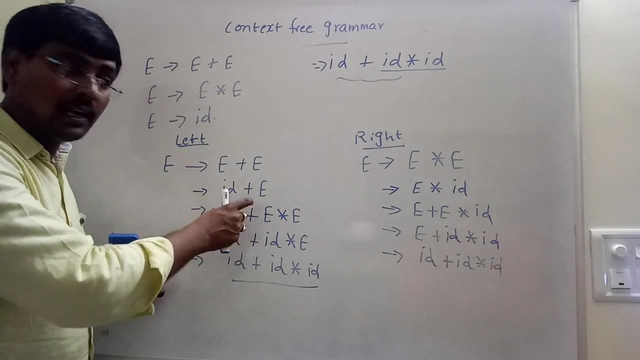 Finally, id plus id into id. This is the string we are deriving. So for a given string, we have leftmost derivation and rightmost derivation. These are the derivations. Now we are going to parse tree. That is the syntax analysis phrase. Simple terms, Parse tree is a pictorial. 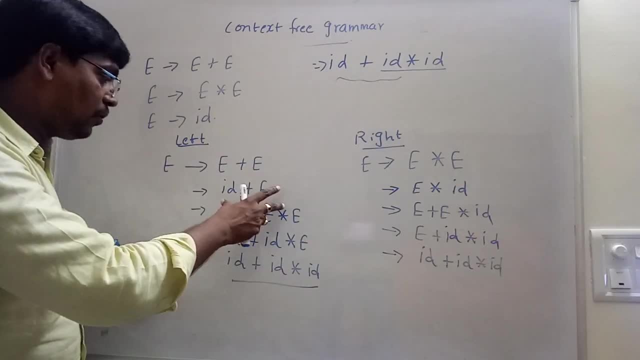 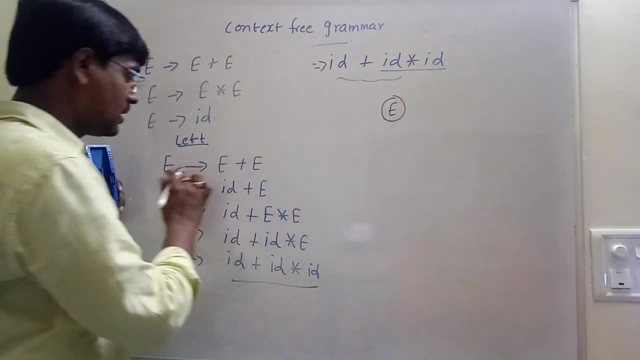 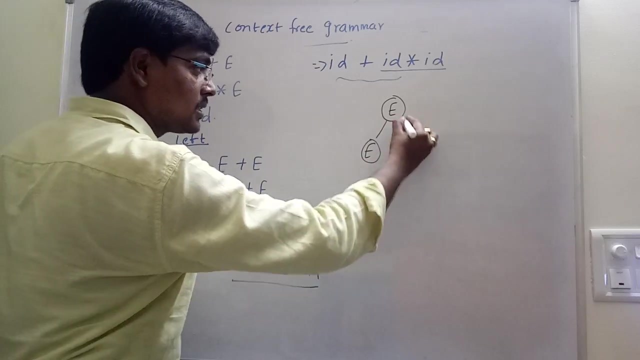 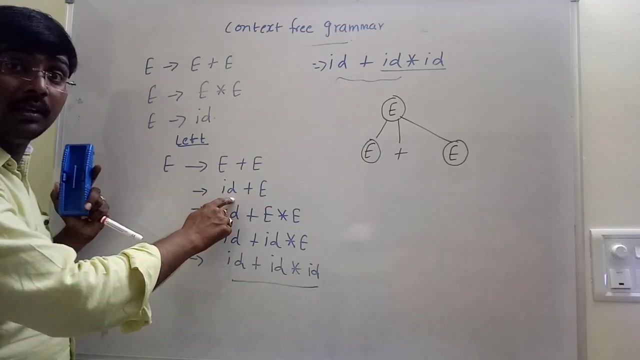 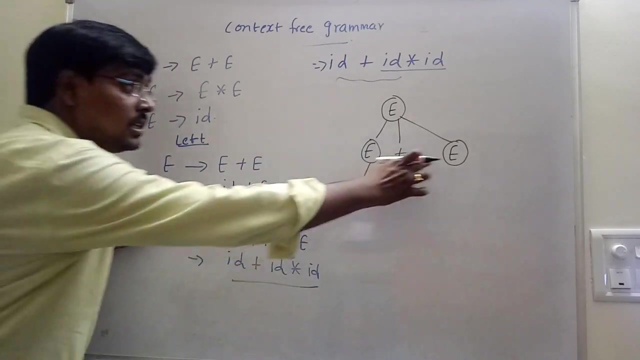 representation of a derivation Suppose for this grammar we are writing. we are writing for constructing the parse tree. So e is the parent node. Now e has two terms: e plus e. Now this e is replaced with id. This e is replaced with id In the next step, this: 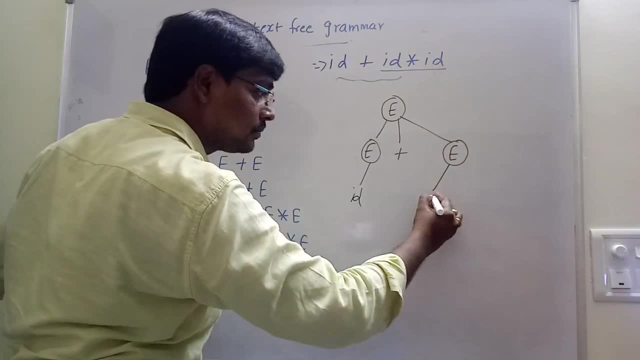 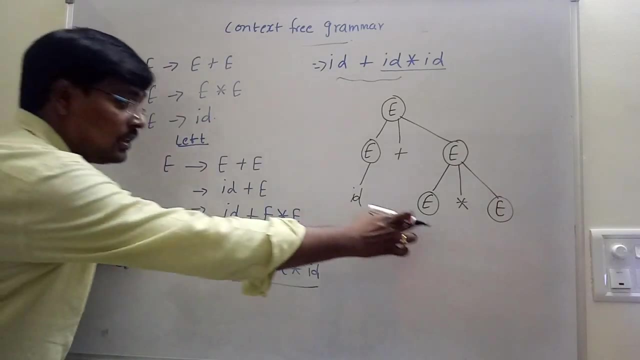 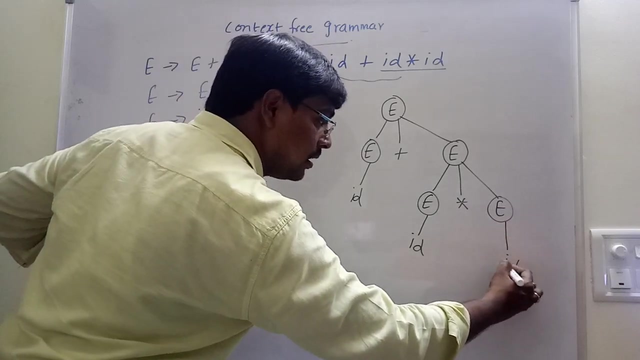 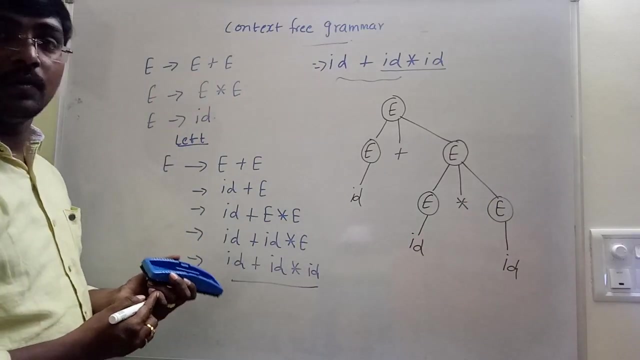 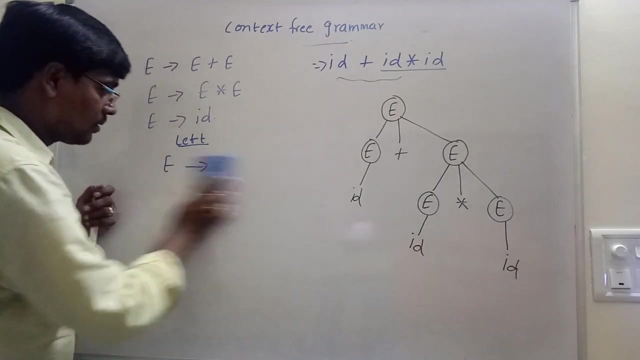 e is replaced with e and e. In the next step, this e is replaced with id. Finally, we are getting the grammar ed plus id into id. Similarly for rightmost derivation also, we are constructing the same parse tree. For example, we have already constructed the rightmost derivation. Again, check the. 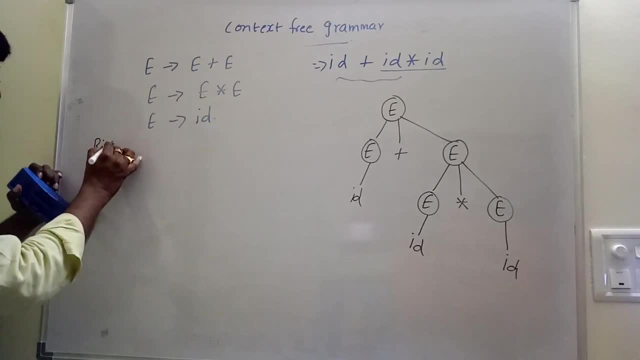 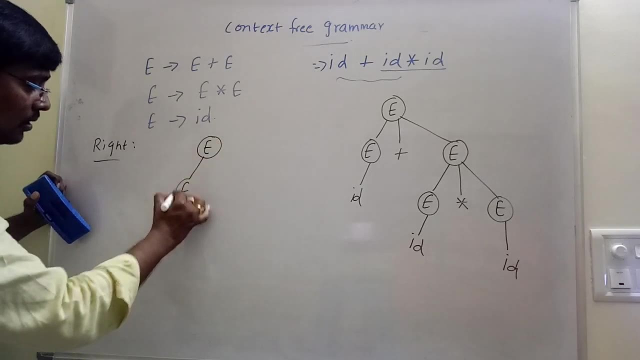 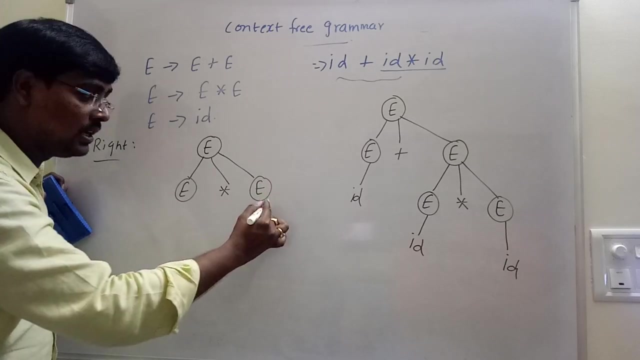 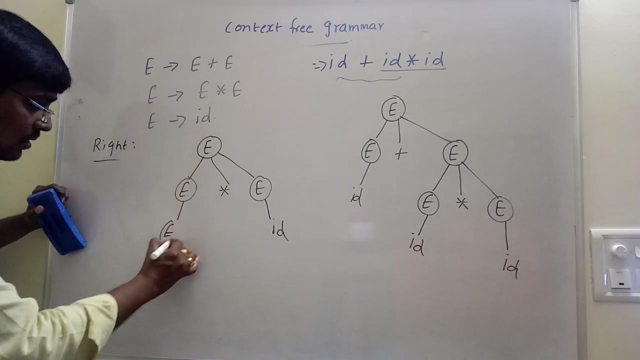 grammar. Again, check the rightmost derivation First of e. now e is constructed into e, into e. In the rightmost derivation first, this e is replaced. This e is replaced with id. In the next step, this e is replaced with e plus e. In the next iteration, this e is replaced. 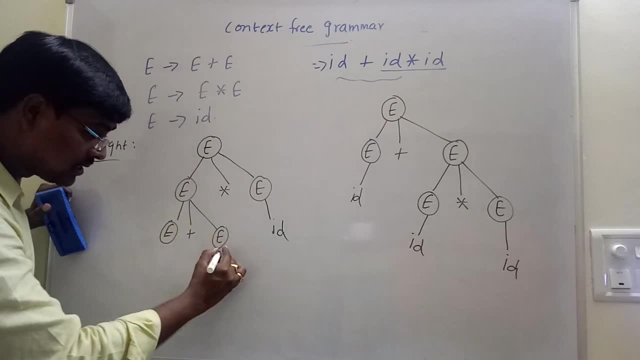 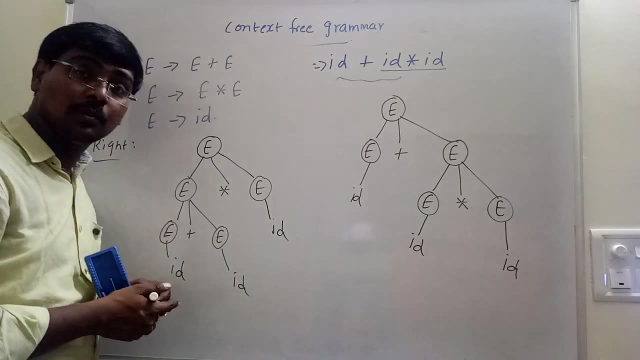 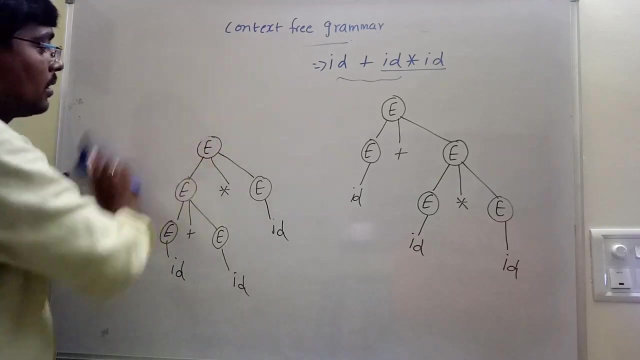 with id. Again checking the rightmost derivation. Again checking noggin. this e is replaced, replaced with id. in next iteration this e is replaced with id. so write step by step procedure. so this is the leftmost derivation, this is rightmost derivation. now check what is ambiguous. 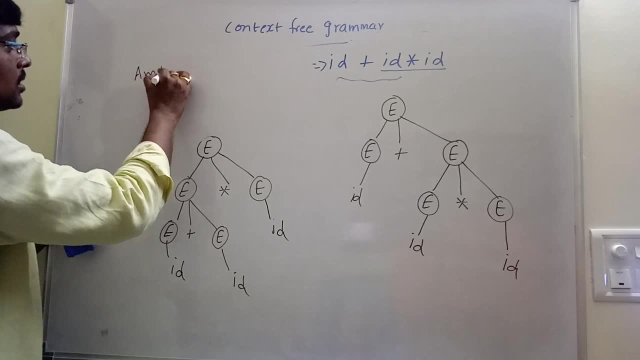 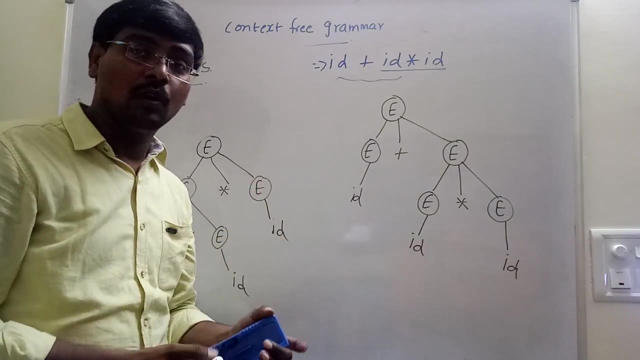 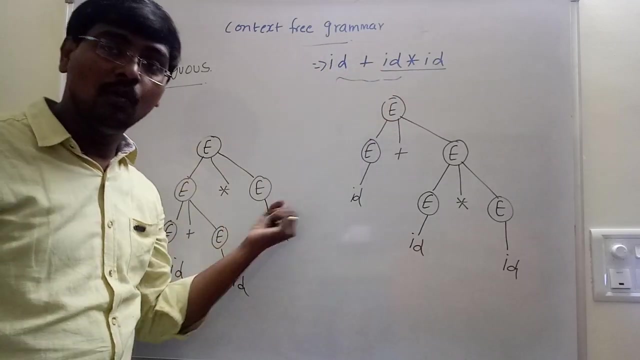 grammar. so ambiguous grammar means if a grammar contains more than one pass tree for a given string. for example, this is the string we want to derive for this string we have more than one pass tree. suppose this is one pass tree for derivation of some string? similarly, this is: 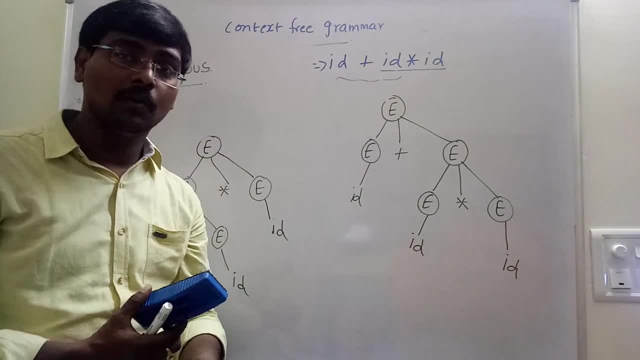 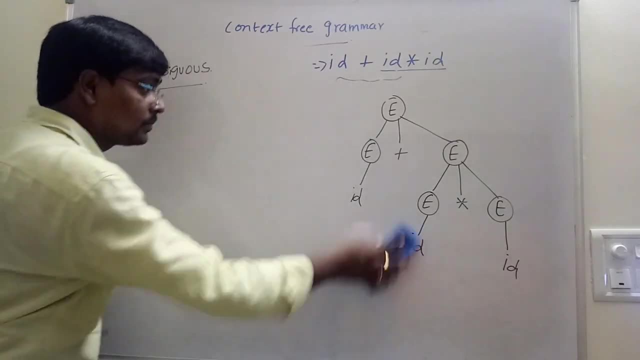 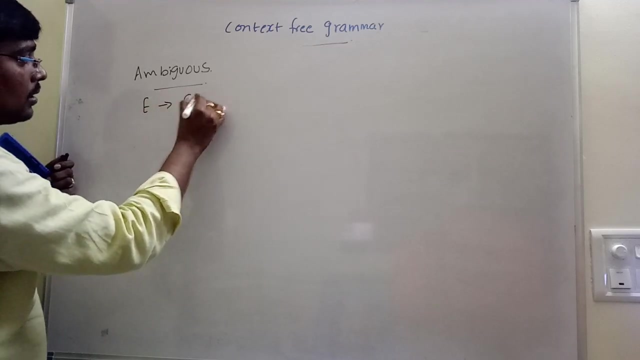 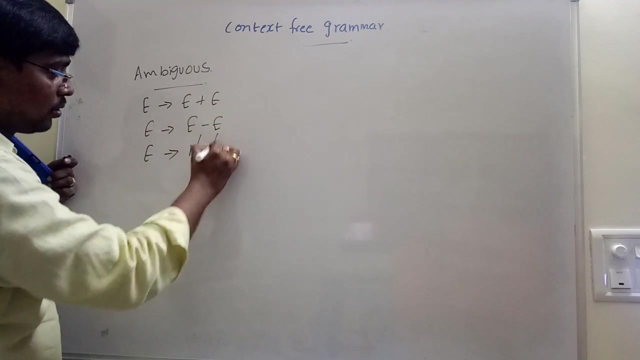 the pass tree for derivation of this string for a given grammar. if we have more than one pass tree, that is called ambiguous grammar. check one more example. suppose, if the grammar is e tends to e plus e, e tends to e minus e. suppose e tends to one, two, three and so on, nine for example. this is the. 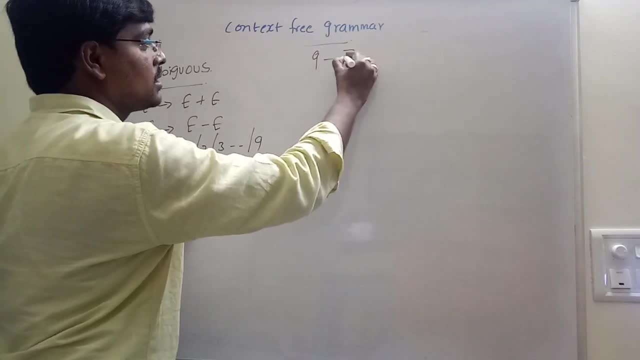 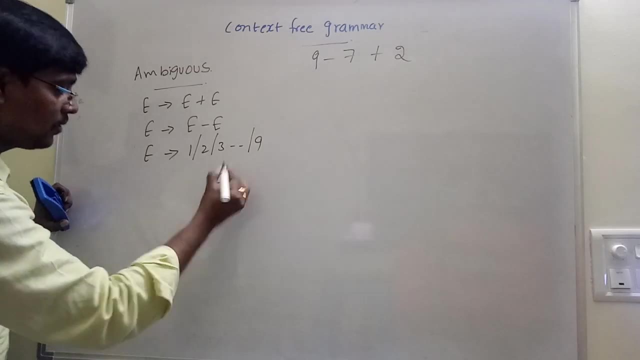 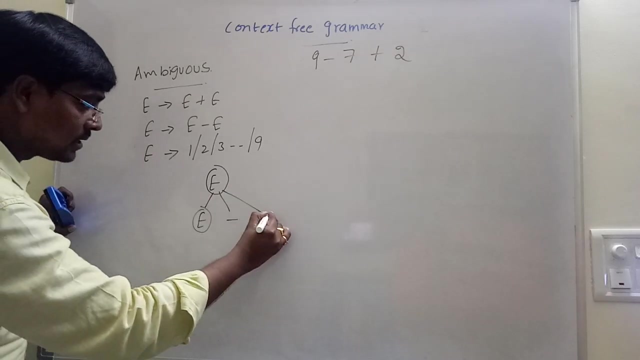 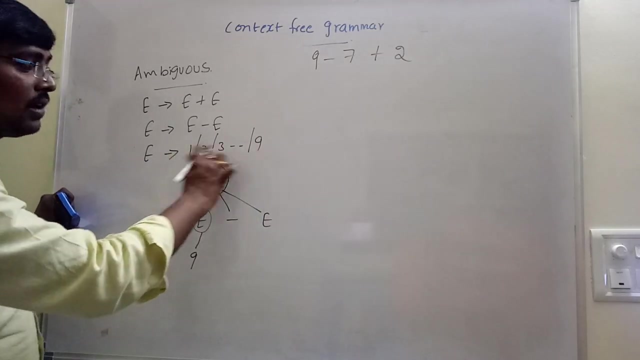 grammar and we want the string some nine minus seven plus two, for example. this is the string we are going to derive first to perform one type of derivation. now e, e is converted into e minus e. e is variable, into e minus e. Now this e is replaced with any value between 1 to 9.. Our required 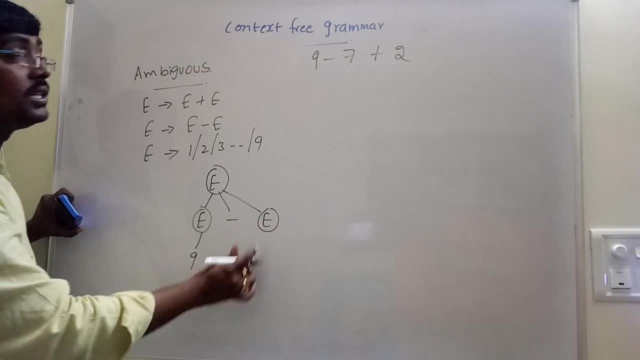 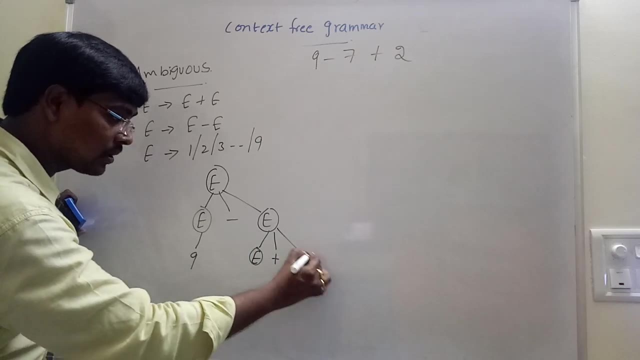 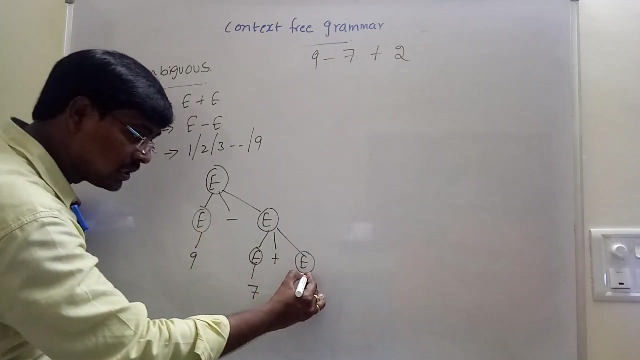 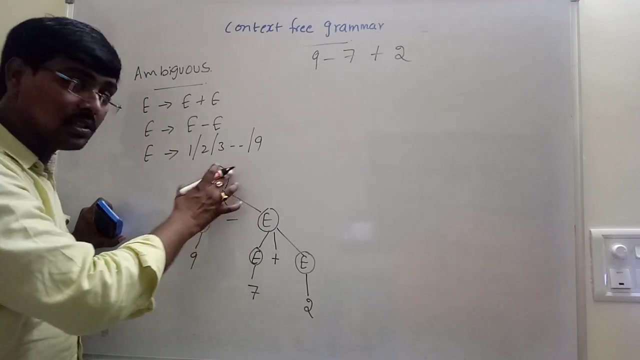 value is 9.. So 9.. Now in the next step, this e is replaced with e plus e. So in the next step, this e is replaced with our value 7.. In the next step, this e is replaced with our value 9.. So here we have to write step-by-step procedure. So positive tree is directly not. 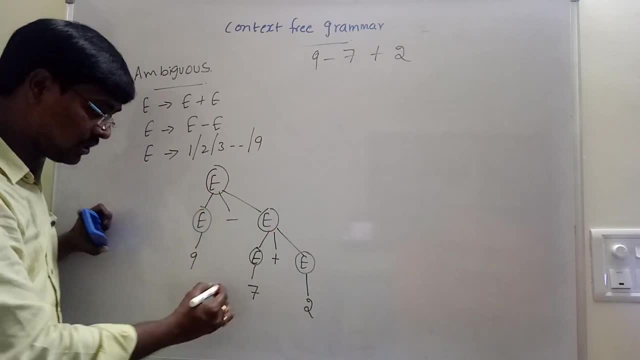 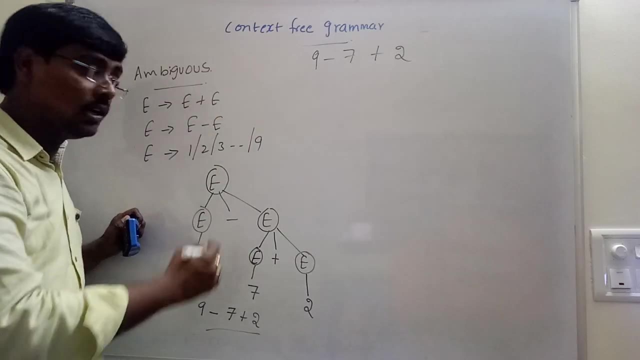 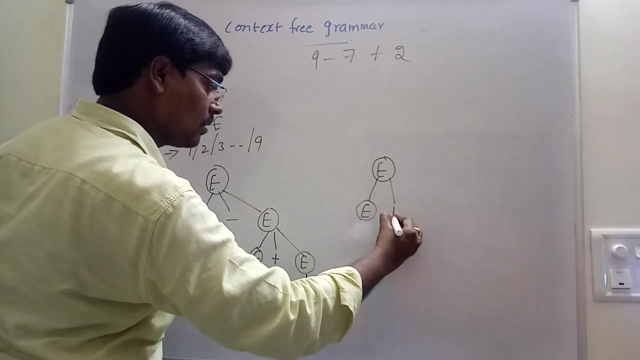 considered the positive tree Step-by-step procedure. we are constructing the positive tree, So the positive tree is 9 minus 7 plus 2.. Suppose for the same string we are constructing one more positive tree. e tends to e plus e. Suppose in this example I am using e minus. 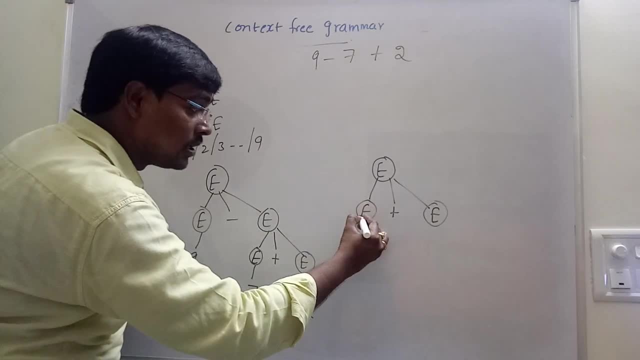 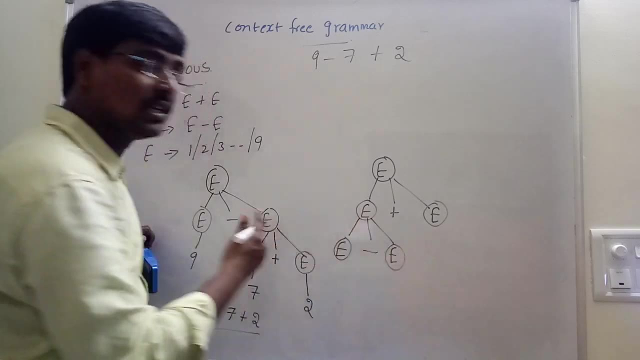 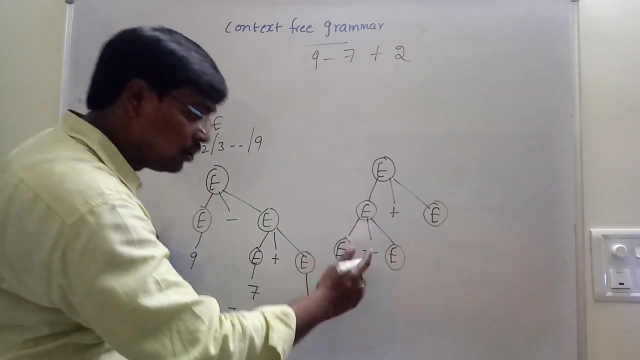 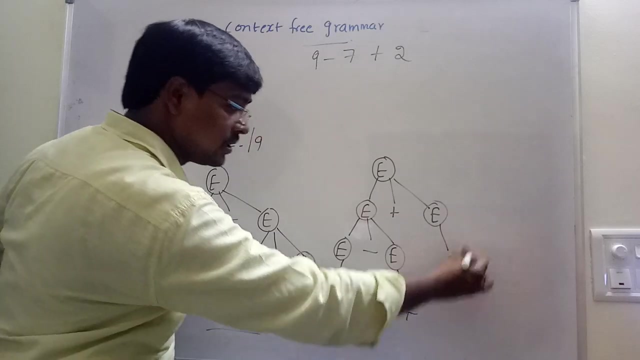 e. Suppose in this example I am using e plus e. Suppose this e is replaced with: in 2 cases I am using leftmost derivation: e minus e and e. So in leftmost derivation now this e is replaced with 9, this e is replaced with 7 and this e is replaced with 2.. So it also. 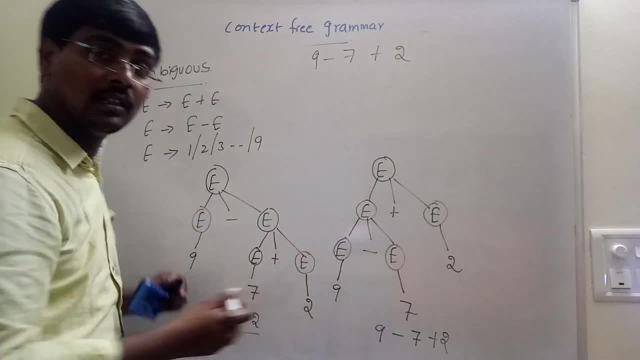 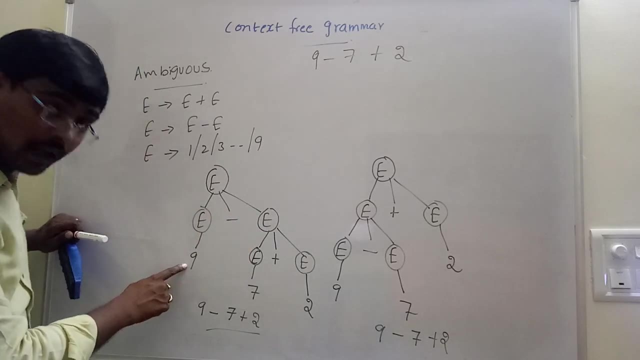 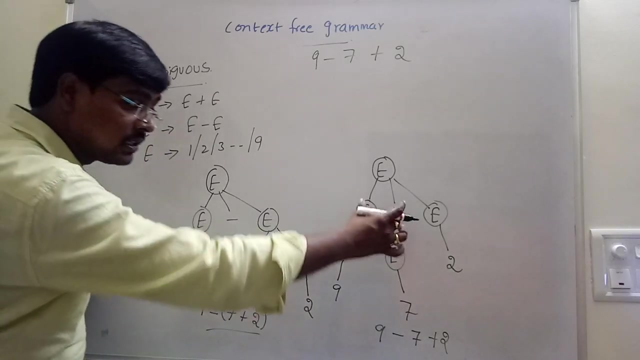 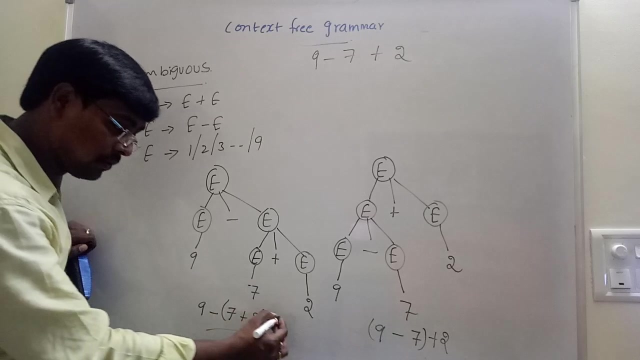 gets 9 minus 7 plus 2.. We are getting the same Here. what is the problem? So in this process, the diagram is 9 minus 7 plus 2. That means 9 minus of 7 plus 2. In this example, 9 minus 7 plus 2. Observe the values: 9 minus of 7. 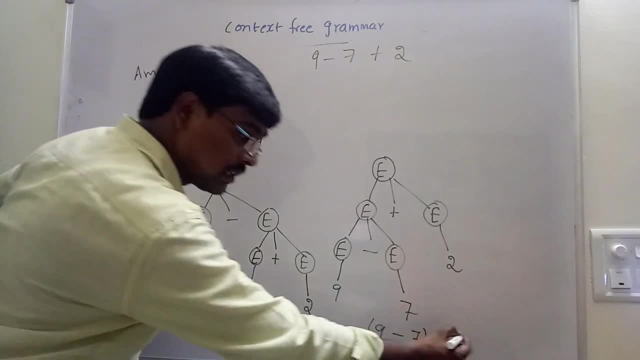 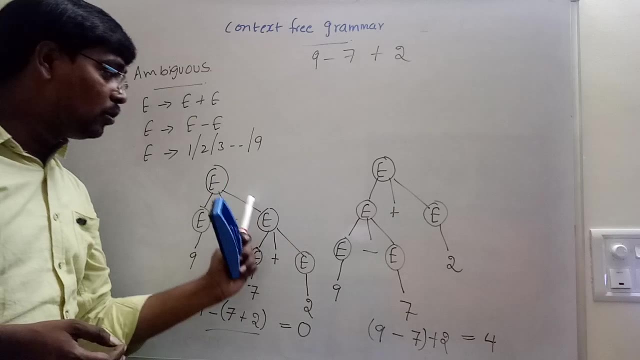 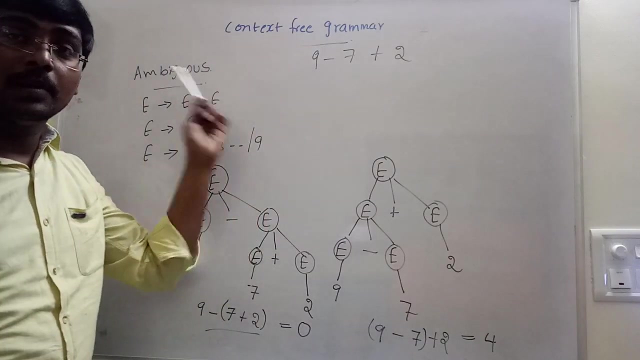 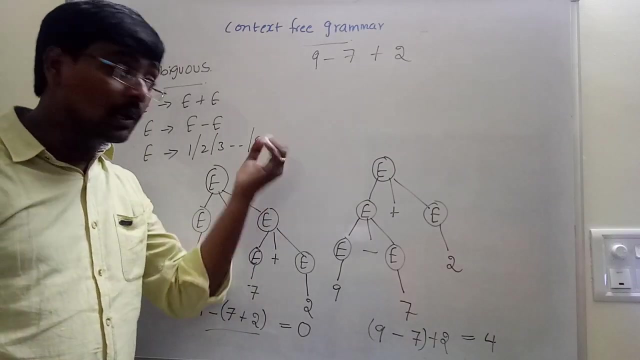 plus 2, it produces 0.. 9 minus of 7 plus 2, it produces value 4.. For the same string, in two types of derivations. for the same grammar, it produces two types of results. So this is ambiguous grammar. So to construct either any positive tree or top-down parser, 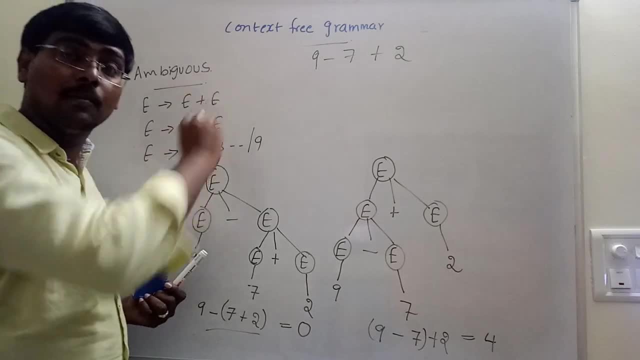 bottom-up parser. the grammar must change. should be unambiguous. Okay, thank you. 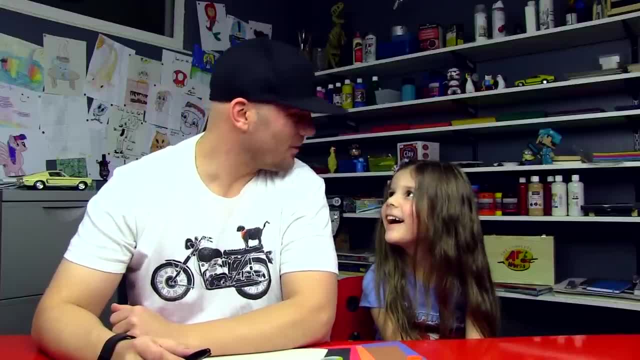 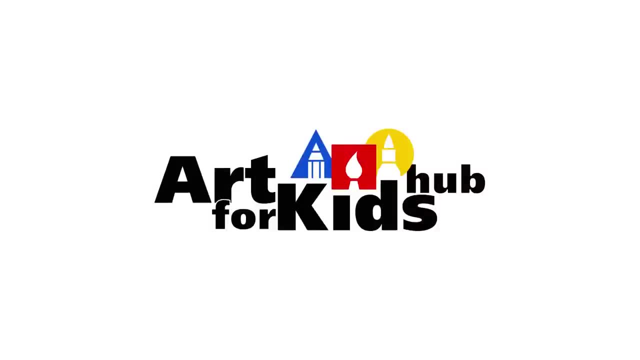 Heads. are we gonna do another winter art project today? Yeah, What are we gonna do? We're gonna do a snowman. Alright, you got your marker. Yeah, Wait, we're gonna need a lot more than a marker, aren't we? Yeah? 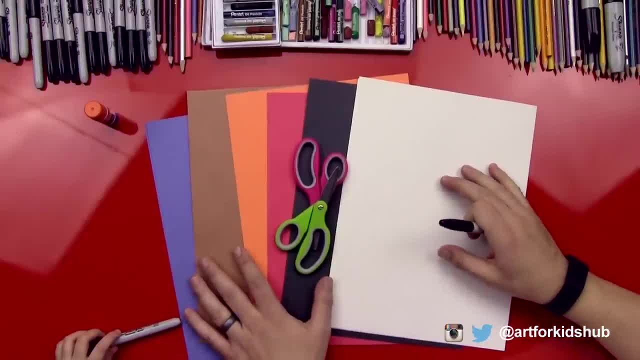 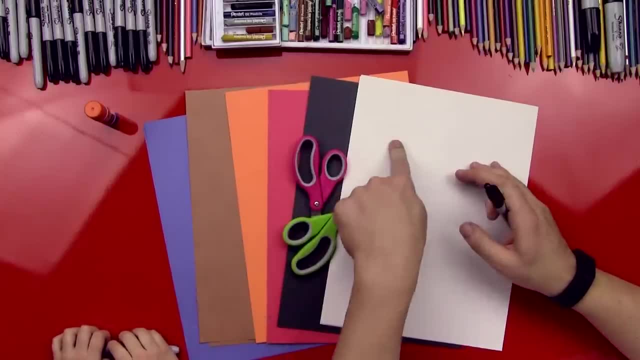 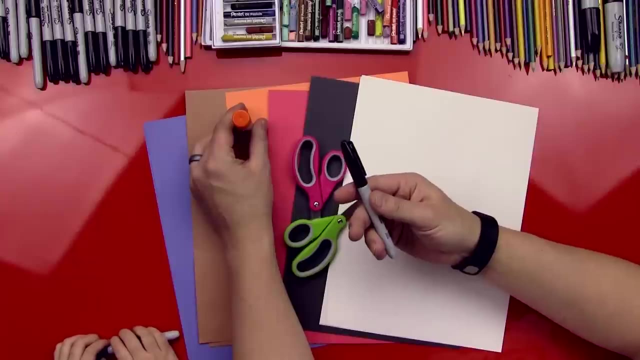 So what's all this stuff? we got here? Paper, Bunch of paper. What colors do we got Blue, Brown, Orange, Red, Black, White, And then we also got scissors, we got some glue and, of course, we got our markers. You ready? 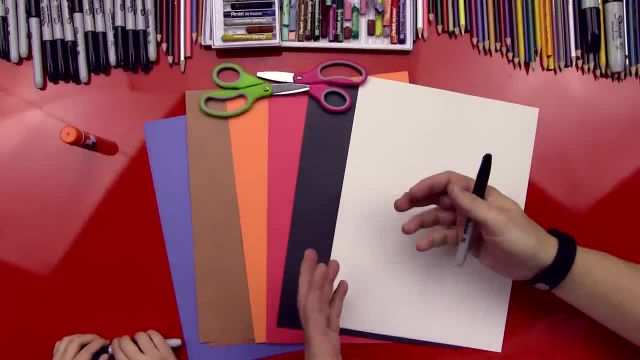 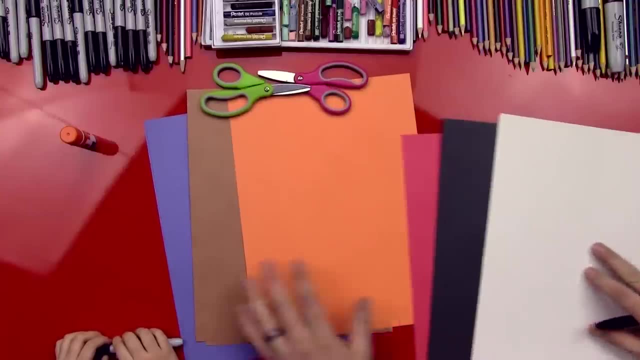 So we're gonna use, we're gonna do a cool drawing, but we're gonna cut it out and glue it all together, Kind of like our roses that we just made. huh, Does that sound like fun? Yeah, Okay, we're gonna first start with the blue and we're gonna use the blue for the background. 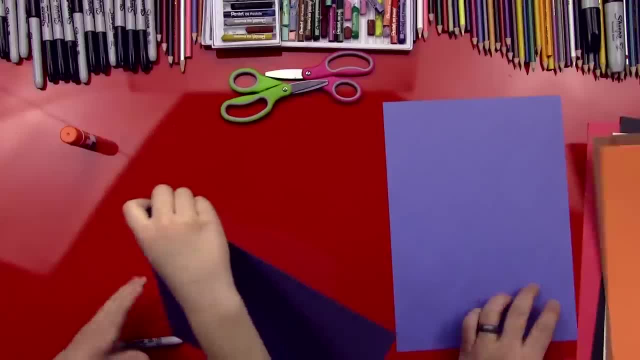 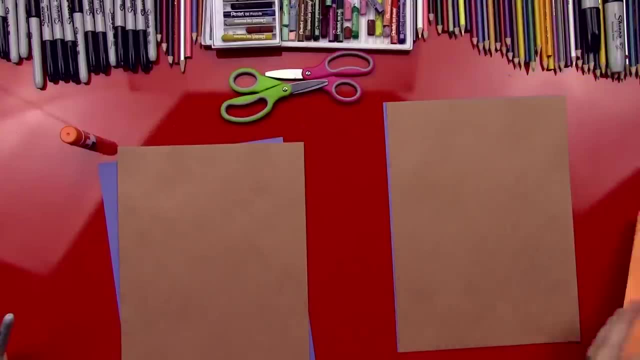 Okay, so grab a sheet of blue and then we're gonna use the brown and we're gonna put the brown on top Like this: Okay, And we're using the brown because what does the snowman have for his arms? Sticks. Yeah, he has sticks.